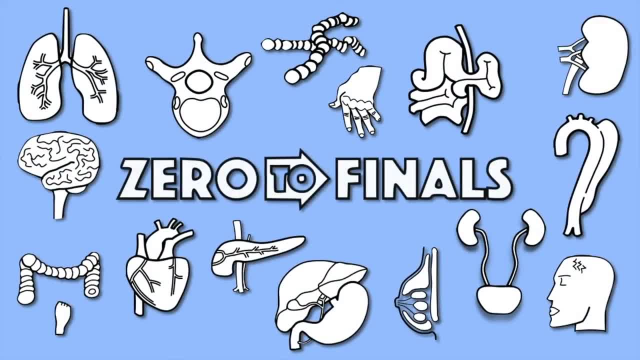 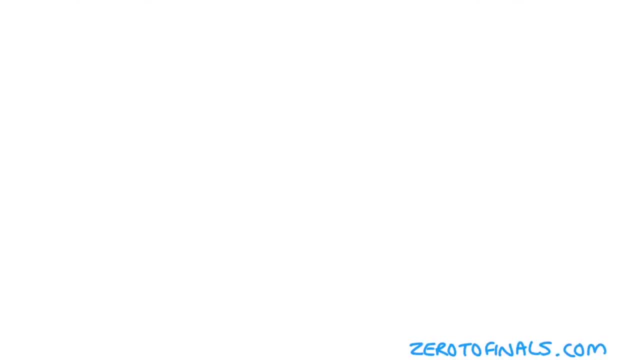 Hi, this is Tom from ZeroToFinalscom. Today I'm going to talk about a concept called Mendelian Inheritance, and specifically the inheritance of autosomal recessive and autosomal dominant conditions. So some genetic conditions exhibit a simple inheritance pattern called 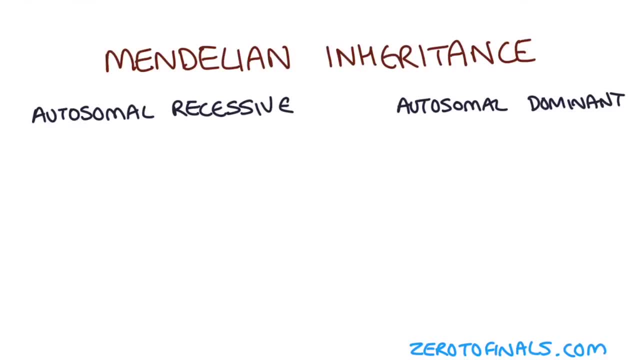 Mendelian Inheritance. This inheritance only occurs where the disease is caused by a single abnormal gene on one of the non-sex chromosomes. So this is the chromosomes that are not the X or Y chromosome. So these chromosomes are called the autosomes. Two examples of diseases: 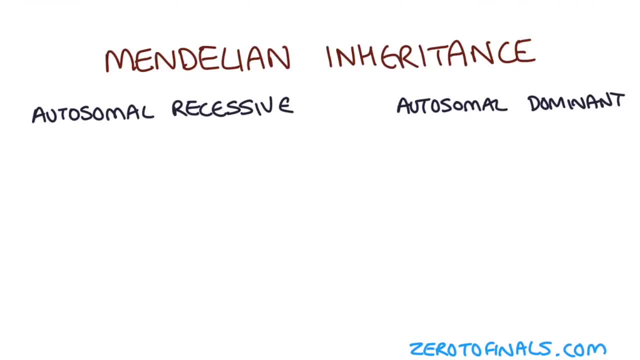 that are caused by a single gene passed on from somebody's parents are Huntington's career and cystic fibrosis. So the difference between these two conditions is that the gene for Huntington's career is dominant over a normal gene And the gene for cystic fibrosis is recessive over a normal gene. So this basically means 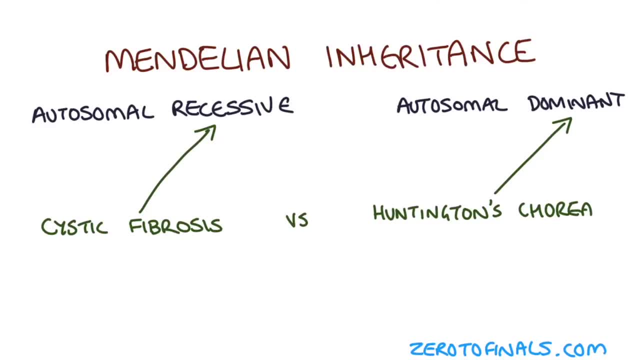 that in order to have the disease of Huntington's career, you only need a single copy of the disease gene, because it will override the other copy of the gene that you have. that's normal, Whereas in order to have the disease of cystic fibrosis, both of your copies of 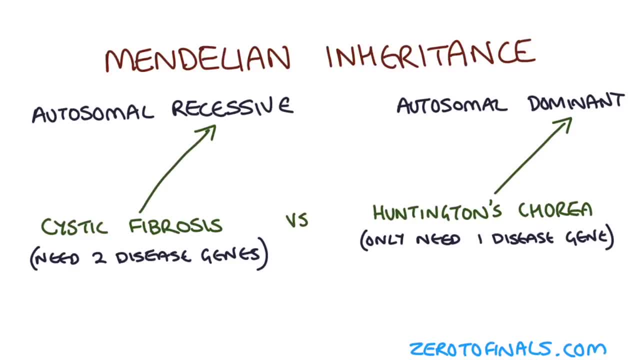 the gene need to be the disease gene, Because if you only have one disease copy, the other one you have, which is normal, will override the disease copy. In this scenario, you're called a carrier because you don't actually have the disease, but you do have the capacity. 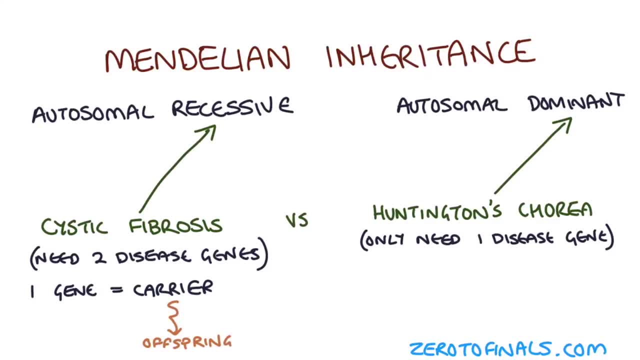 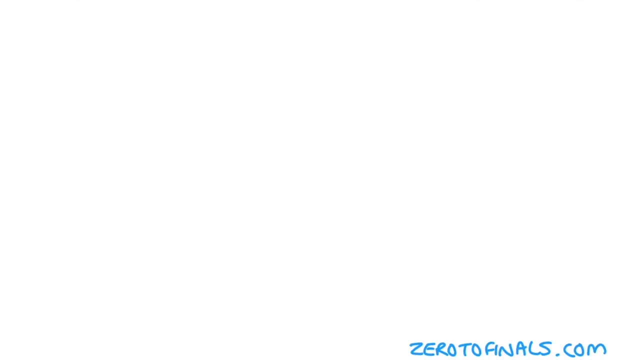 to pass it on to your offspring. So we refer to diseases like cystic fibrosis as autosomal recessive and diseases like Huntington's as autosomal dominant. So now I'm going to go through how you actually calculate the risk of one of the offspring. 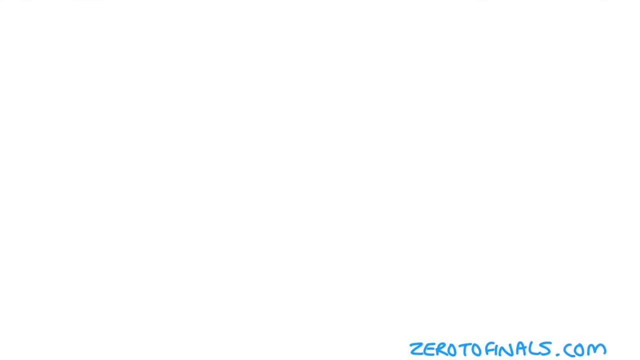 passing on an autosomal recessive condition. So, in order to calculate the risk of passing on an autosomal recessive condition, it's really helpful to draw out an inheritance pathway. By using this method, you can always work out the risk of various outcomes based. 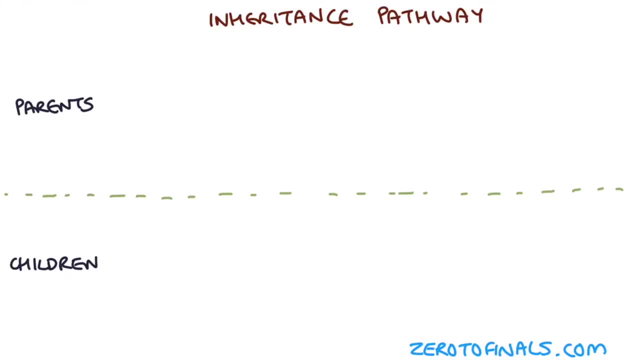 on the genetic status of the parents. So I'm going to use some examples in order to demonstrate this method that could help you in your exams and also in explaining things to parents in real life practice. Firstly, let's consider: both parents are carriers of an autosomal recessive condition. 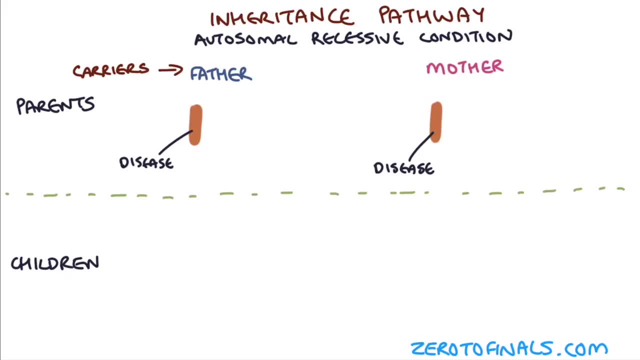 Each parent has one disease gene and one normal gene And, as a result, they do not have the disease, but they do have the potential to pass the disease on to their children. So let's label the copies of the gene that could be inherited from the parents as copy 1 and. 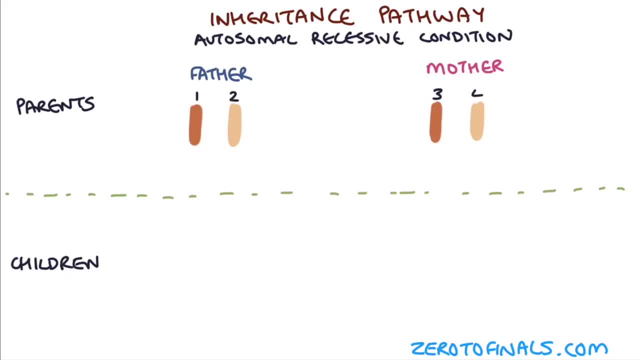 copy 2 from the first parent And, as a result, they get the disease gene of copy 1 from the father and copy 3 and copy 4 from the mother. There's always 4 possible outcomes to the inheritance of this specific gene. 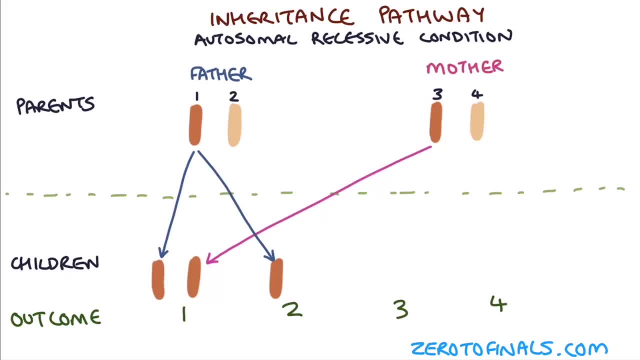 Outcome 1 is copy 1 from the father and copy 3 from the mother. Outcome 2 is copy 1 from the father and copy 4 from the mother. Outcome 3 is copy 2 from the father and copy 3 from the mother. 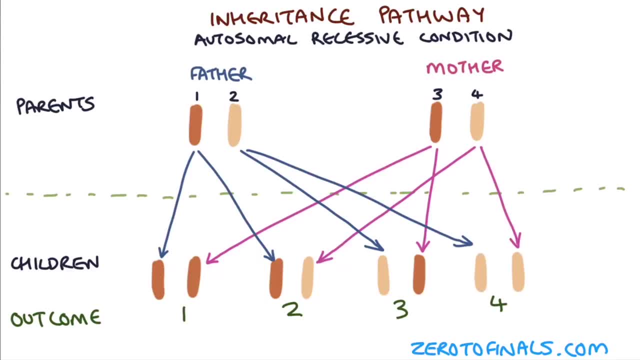 from the father and copy four from the mother. So let's say copy one and copy three are the autosomal recessive disease genes and copy two and copy four are normal genes. So outcome: one has two copies of the gene that codes for the disease and therefore this person would have the 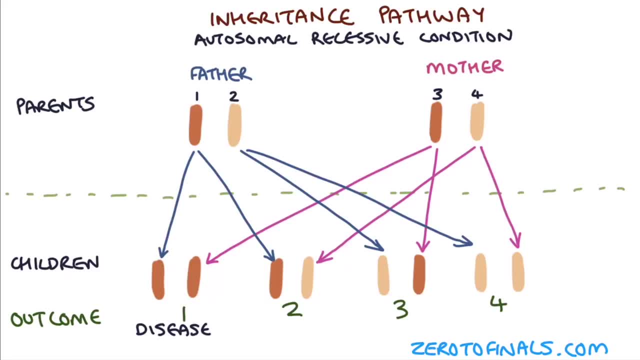 disease. So outcome two has one copy that codes for the disease and one normal copy, and therefore this person is a carrier, just like their parents. Now outcome three again has one copy that codes for the disease and one normal copy, and therefore they're a carrier as well. Now outcome four has: 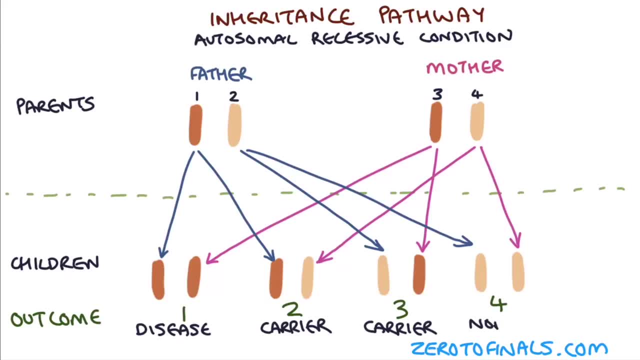 two normal copies of the gene and therefore is free from the abnormal gene and doesn't have the disease and is not a carrier. Therefore, the children of these parents have a one in four chance, or 25% chance, of having the disease, a two in four or 50% chance of being a carrier and a one in four or 25% chance of having 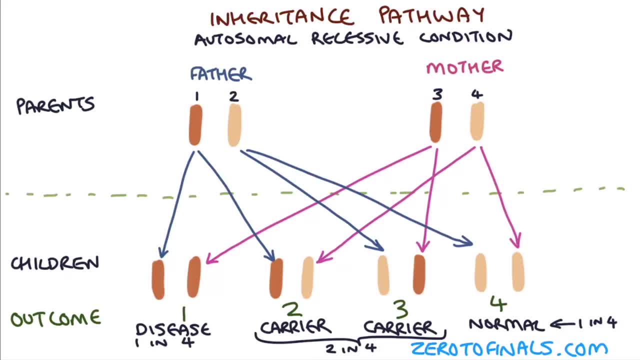 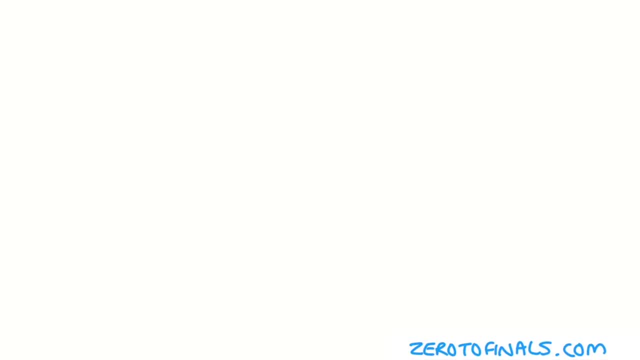 normal genes. So by doing this, you can calculate quite easily the risk of the children either having the disease, being a carrier or having normal genes. So now, finally, I want to give one scenario that illustrates calculating the risk of passing on an autosomal dominant condition. We can use the same method that we did for autosomal recessive. 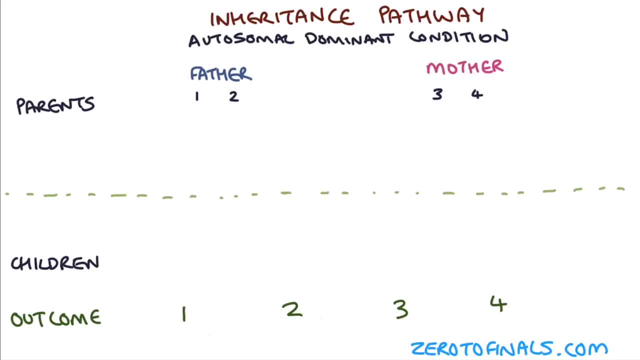 conditions. So, for example, let's say we want to know the possible outcomes where one parent has a condition and the other parent is disease free. We need to know whether the affected parent has one or two copies of the gene for the disease, because either way they'll have the condition. 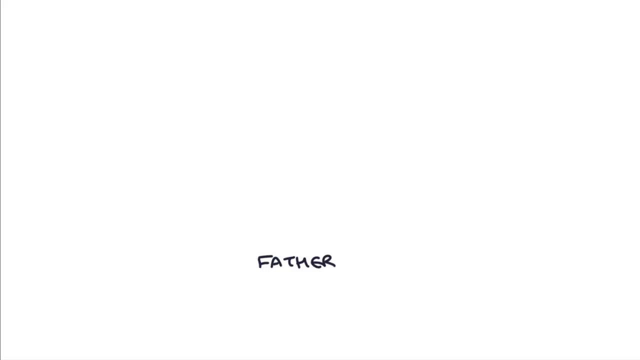 So we can do this out through either genetic testing or asking about the affected parent's own parents. If the affected person had one affected parent, we know that they only have one copy of the disease gene. However, if they had two affected parents, it's possible that they also could have. 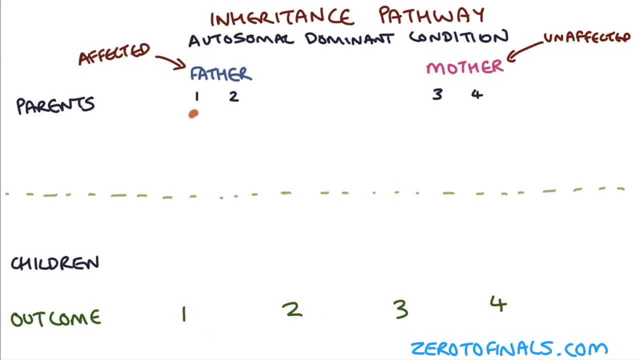 two copies of the disease gene. So for this example, let's assume they only have one copy of the disease gene. So again, we start with four copies of the gene, two from each parents, and let's assume that copy one is the gene for the disease Outcome. one is copy one and copy three. 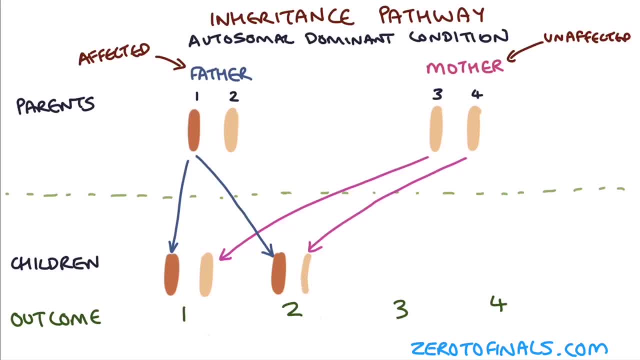 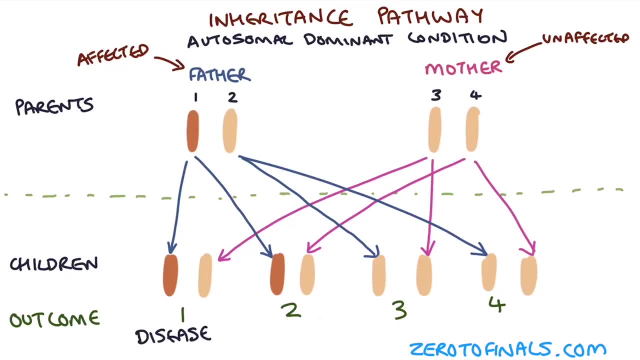 Outcome two is copy one and copy four, Outcome three is copy two and copy three and outcome four is copy two and copy four. So therefore, outcome one has the disease, outcome two has the disease, outcome three has two normal genes and outcome four has two normal genes. So therefore, the children of these parents have a two in four. 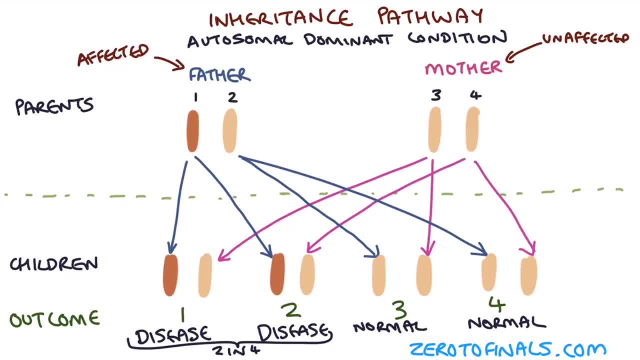 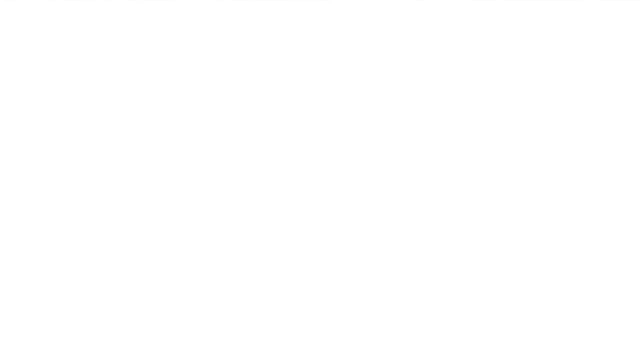 or fifty percent chance of having the disease and a two in four or fifty percent chance of having normal genes. So I hope this explanation has made it a lot clearer about how you calculate the inheritance of these single gene diseases. If you'd like any more information or you're a bit confused, 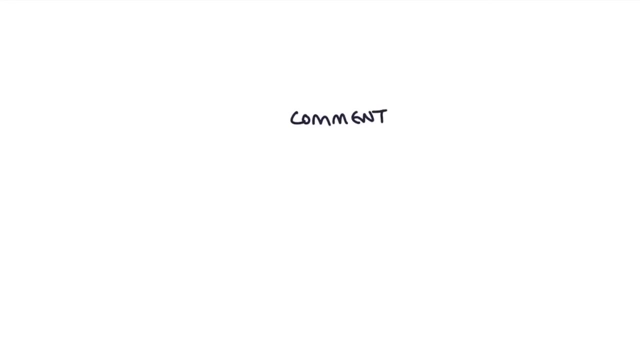 please post in the comments below. I'd be really grateful if you could like this video, subscribe to the channel for more videos and also check out the Xerodefinals website, where there's loads of resources at xerodefinalscom, and I'll see you next time.